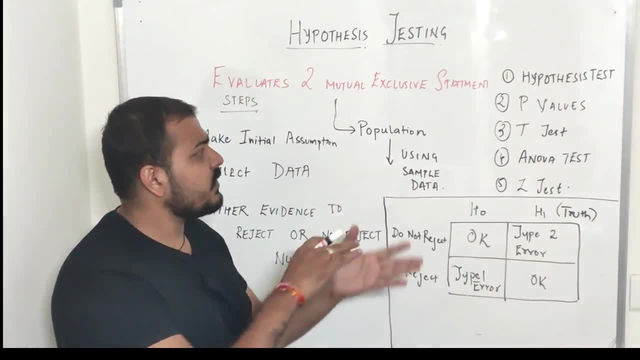 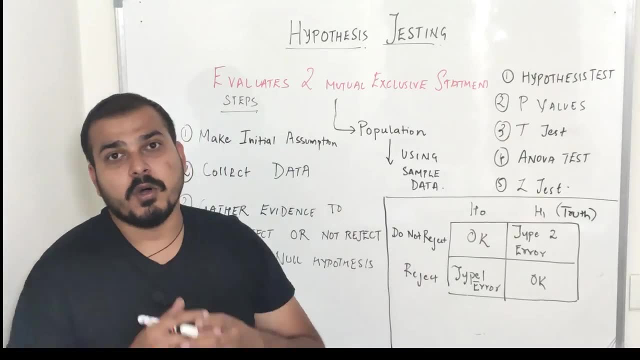 Type 1 and Type 2 Error. So in the upcoming videos, in around 3 to 4 videos, we will complete this whole thing about Hypothesis Testing so that you will not be having any questions furthermore. So let us go ahead. What exactly is Hypothesis Testing? 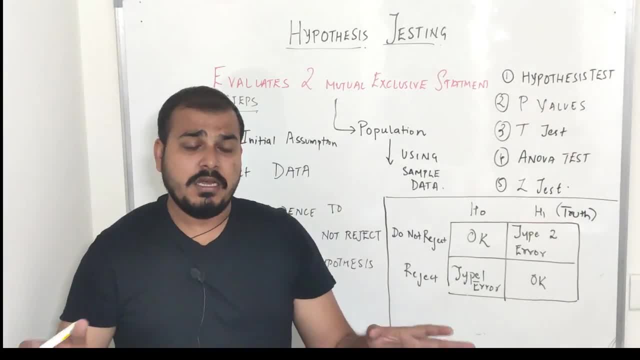 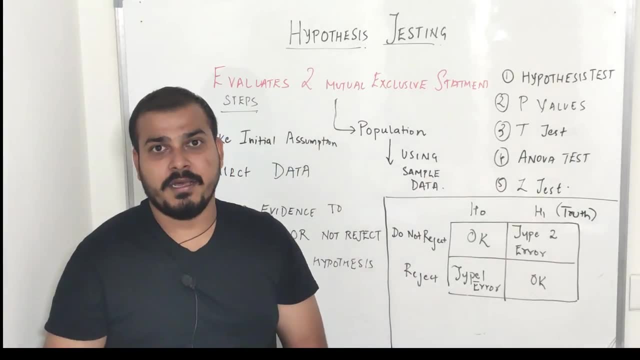 See guys, statistics is all about data. There is a huge amount of data, and that data will only be useful if you are going to analyze it, if you are going to find out some conclusions from it. So it is very, very much important. 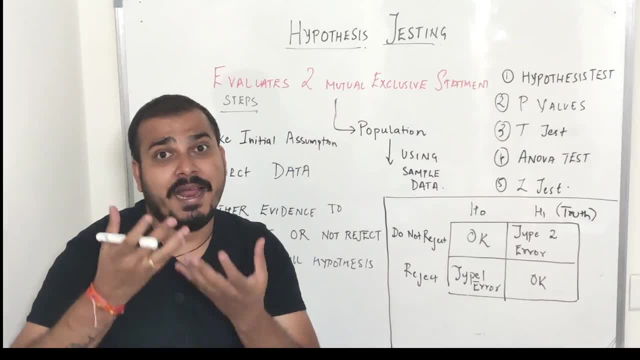 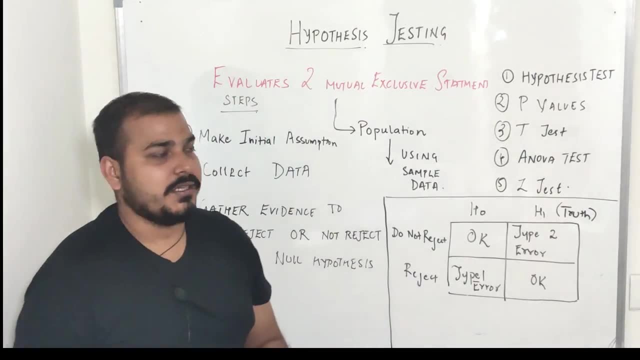 And to find out such important interpretation and conclusion, we basically use Hypothesis Testing. Now, generally, what is exactly Hypothesis Testing? We will discuss about that. what is Hypothesis Testing? What are the different types of Hypothesis Testing? What are the steps in Hypothesis Testing? 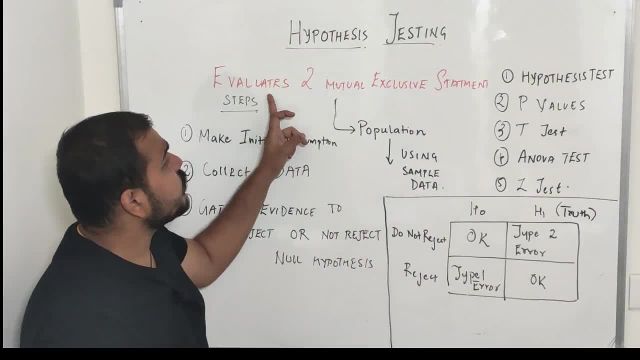 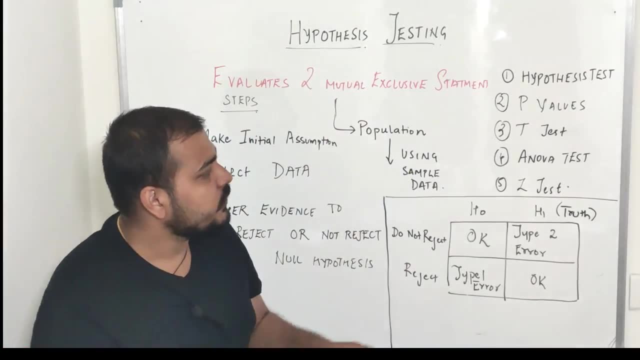 Everything we will try to discuss. So in Hypothesis Testing we actually evaluate 2 mutual exclusive statements, And this is just an example. We can evaluate 3 to 4 mutual statements also. For that we usually use ANOVA Test. 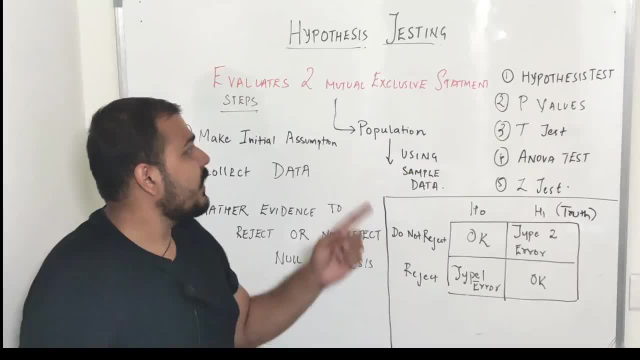 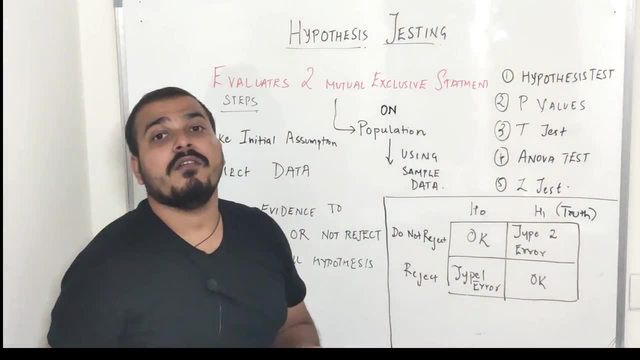 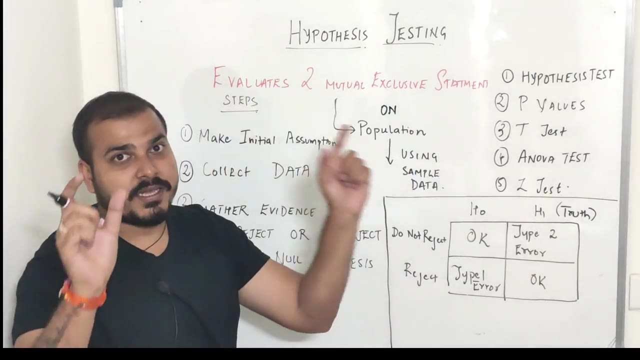 But just understand in the basic terminology. we try to evaluate 2 mutual exclusive statements on a population using a sample of data. Just try to understand this. We evaluate 2 mutual exclusive statements, So there are 2 things. Either this one can be true or this one can be true. 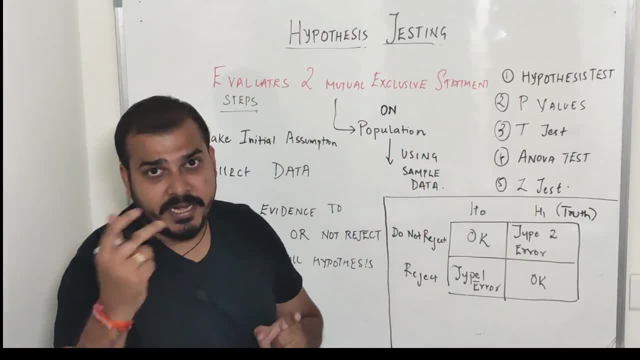 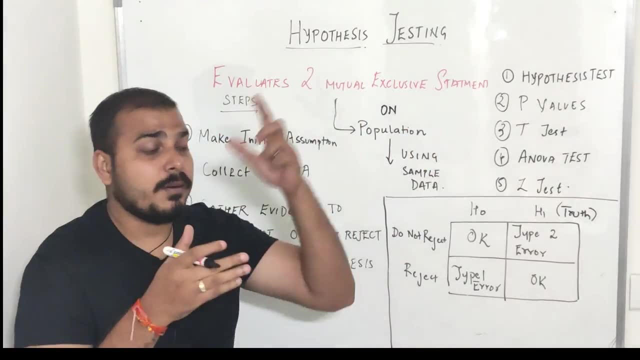 It may be any statement On a population data, using sample data, And then we finally conclude that this population belongs it is true for a particular statement or the other statement. Just think in this particular way. So I may say that I may take a very good example. 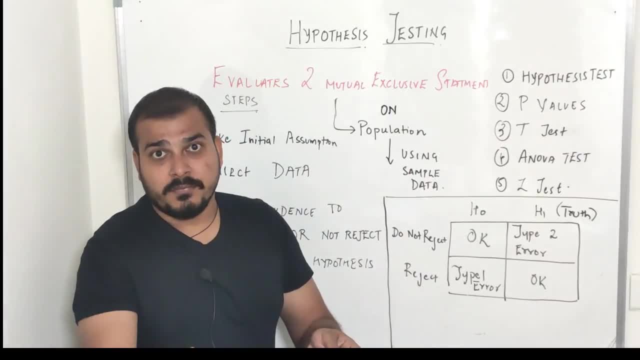 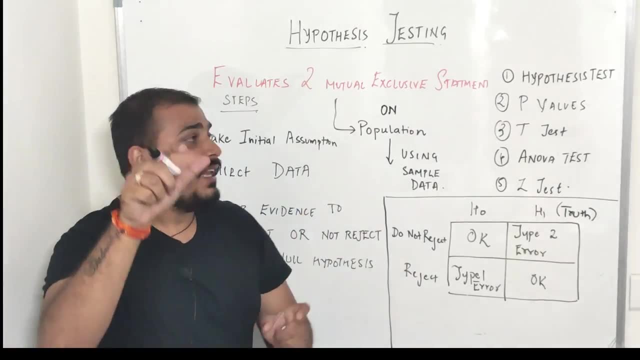 In the court of law. I may say that the defendant is guilty, The defendant is innocent. So these are 2 statements And one of the statement can be true. How it will be true, I will just discuss about the steps And for testing that. 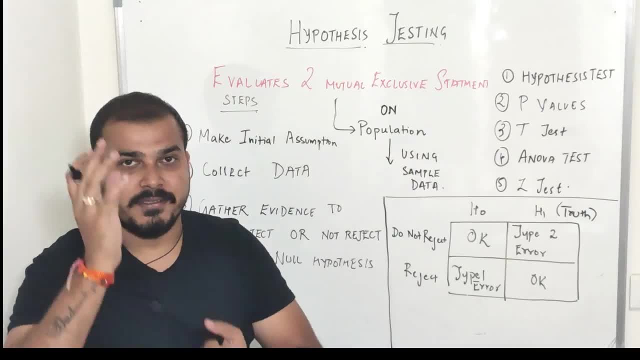 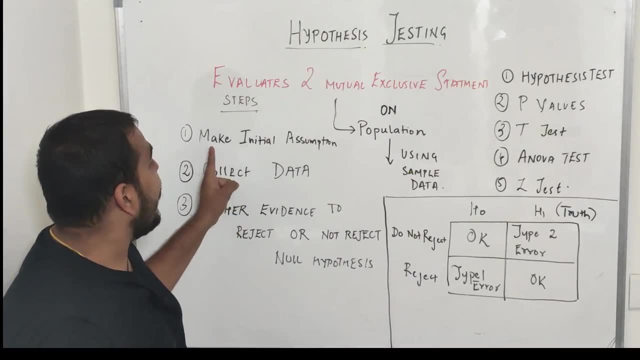 again, guys, for testing that we need evidence, We need evidence. So let us go ahead and take a particular example. What are the steps of Hypothesis Testing? So, over here, the first step says that we have to make an initial assumption. Now, if I take an example, 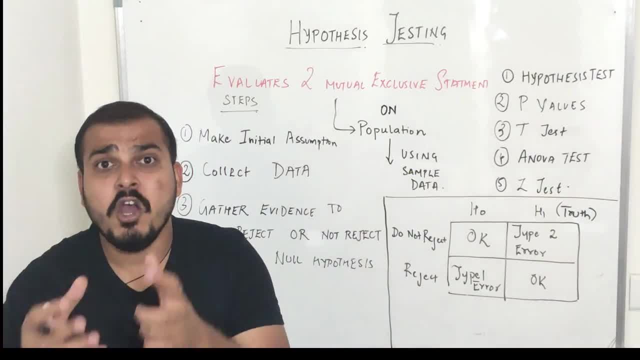 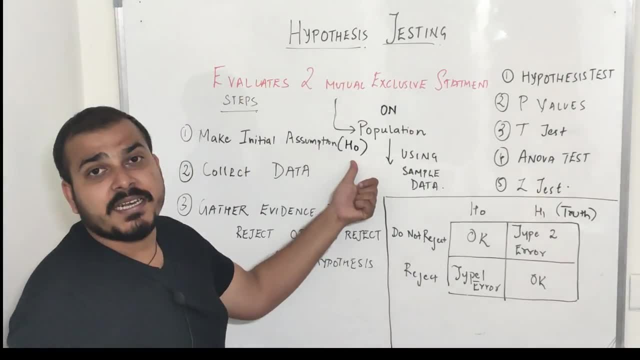 of whether the defendant is guilty or he is innocent. So let me consider that I am taking the initial assumption as H0.. And H0 basically says to me, it is basically called as Null Hypothesis And this H0, I can make an assumption saying that 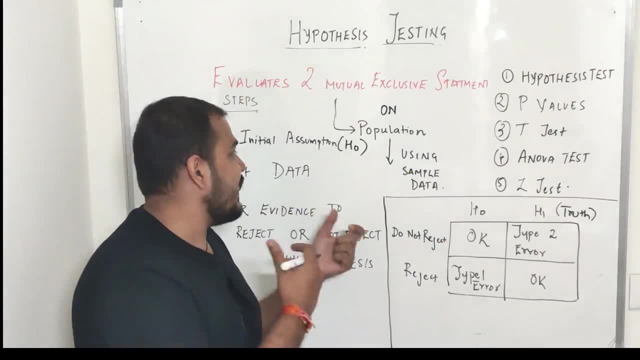 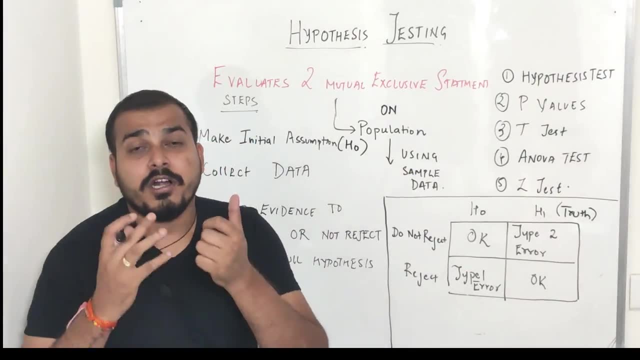 the defendant is innocent. So I will be assigning that particular first statement to this. So I am making an initial assumption. Then I will start collecting the data. Now, what is this particular data? This particular data will nothing be, but it will be just evidences. 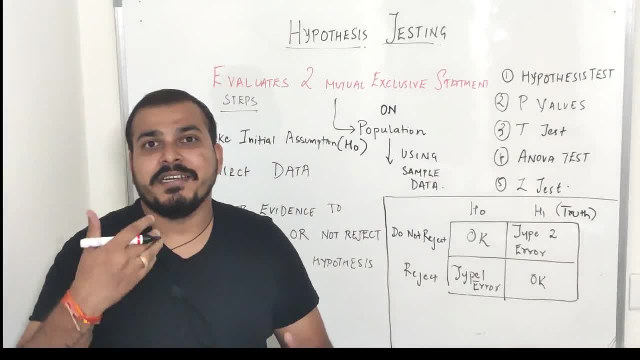 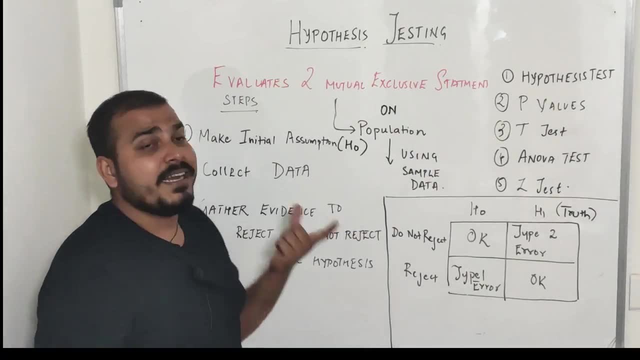 Now for the criminal cases. I may take the finger prints, I may take the DNA prints and lot of things To find out whether the defendant is guilty or whether he is innocent. So I will start collecting the data, which is also called as evidences. 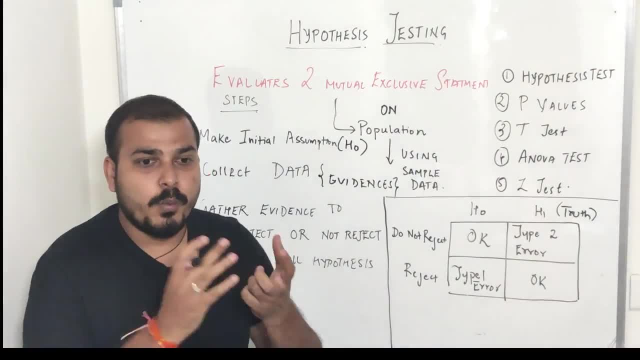 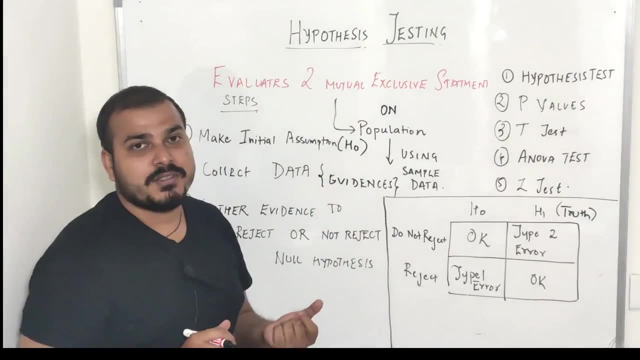 Now I will gather these evidences and then I will try to analyze whether to reject this Null Hypothesis or whether should I accept the Null Hypothesis. Now, in this Null Hypothesis is what? Whether the defendant is innocent or not, 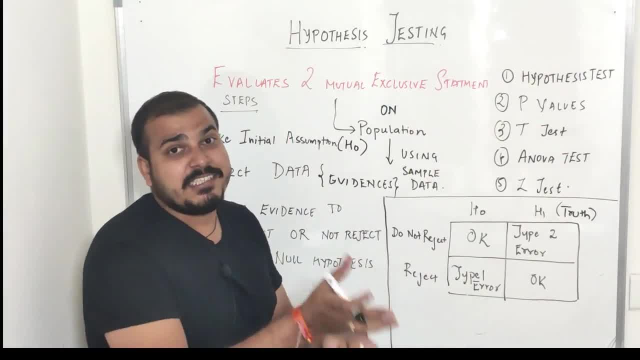 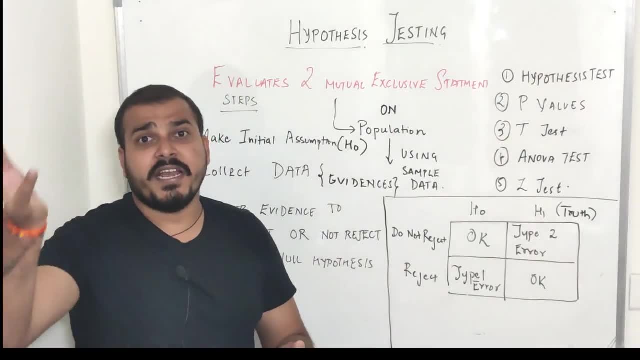 And suppose, if I just take an example of court of law, if the evidence is against him, I will actually reject this and I will say that the defendant is guilty. This is just an example. But in case of data, when we have huge amount of data, 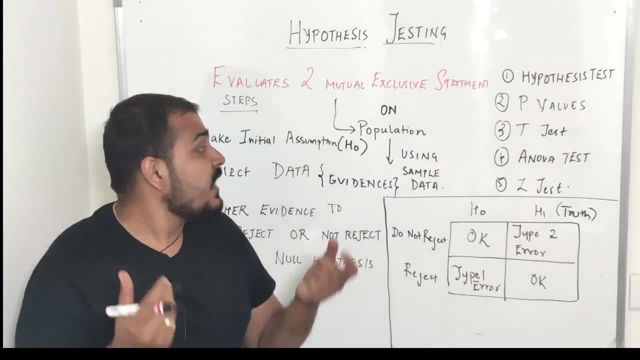 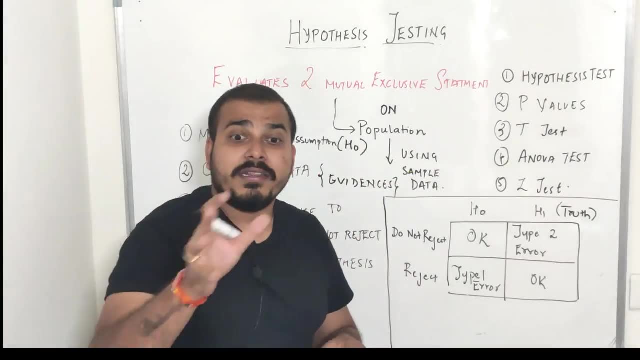 we will try to analyze that particular data, We will try to experiment towards the particular data, considering the sample data, Not the population, but sample data, And then we can actually come to a conclusion on that population, whole data itself. So that is what. 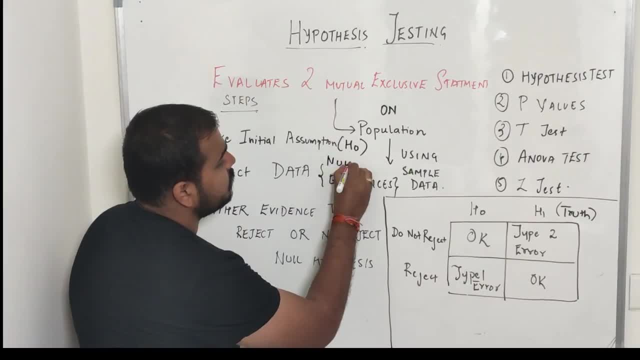 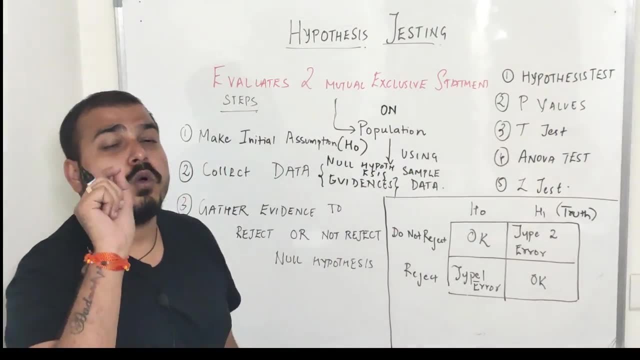 These are very initial steps, guys. This is called as Null Hypothesis, So the defendant is innocent, This becomes a Null Hypothesis. There is also one more hypothesis which is called as Alternate Hypothesis, So we indicate it as H1.. 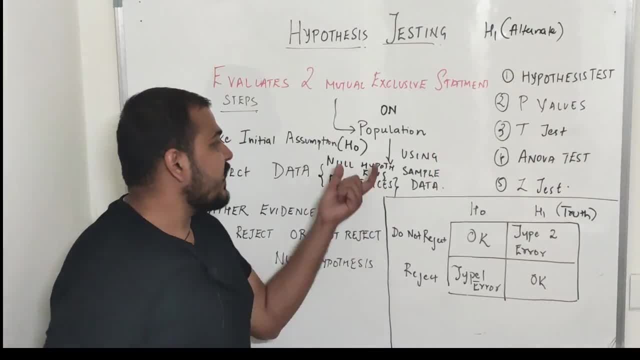 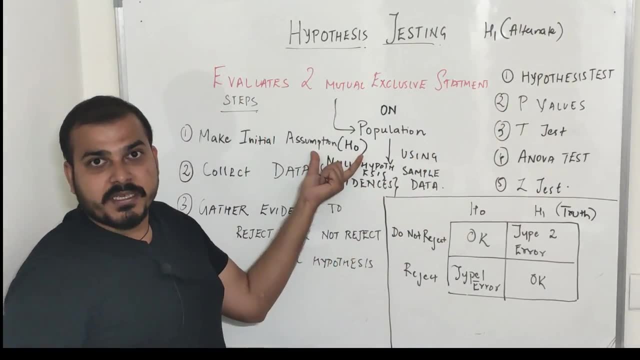 The H1 will be the opposite of H0. So if the defendant is innocent over here, over here, the defendant will be guilty. So if we are able to prove this, then this becomes true. If we are not able to prove this due to the lack of evidences, 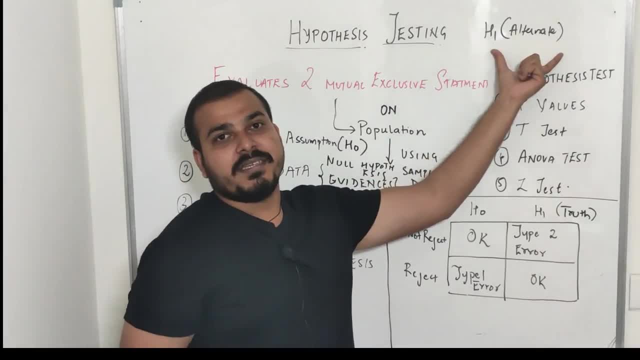 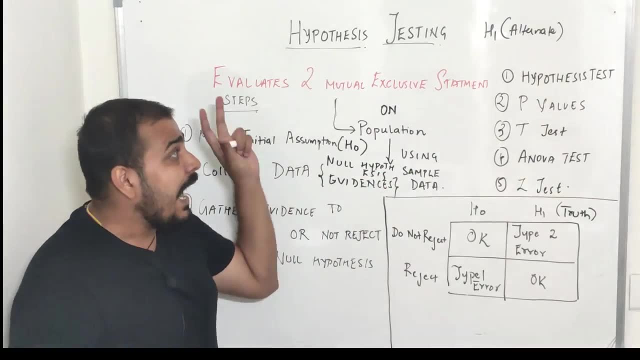 we will actually reject this and accept this Alternate Hypothesis. Pretty much simple, Just considering in this particular way. just understand these basic concepts, guys. How to do it, How to do it mathematically, How to do it with the help of code. 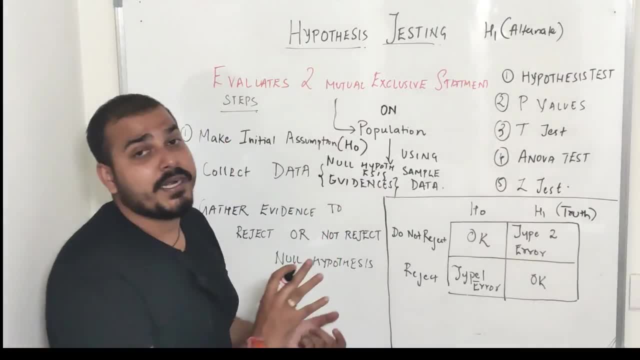 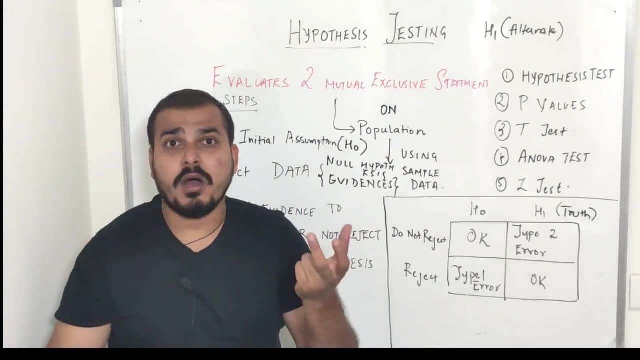 I will be explaining in the upcoming course, But this is very important to understand. what is Null Hypothesis? What is the Alternate Hypothesis? This is the Null Hypothesis. This is just an experiment. The experiment has two outcomes. 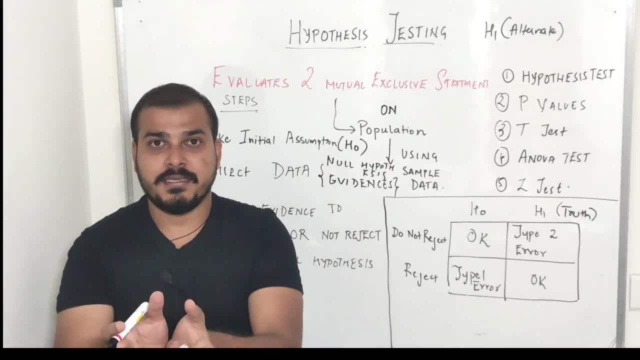 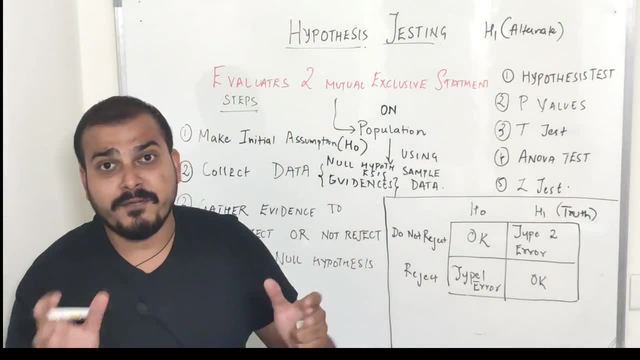 Either one can be true, the other can be true, And for that you have evidences. Whichever evidences supports which either it can support Null Hypothesis or Alternate Hypothesis. So either of them one will be actually true And again we require lot of evidences for that. 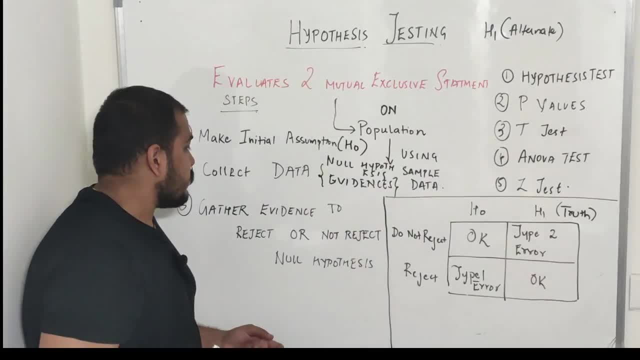 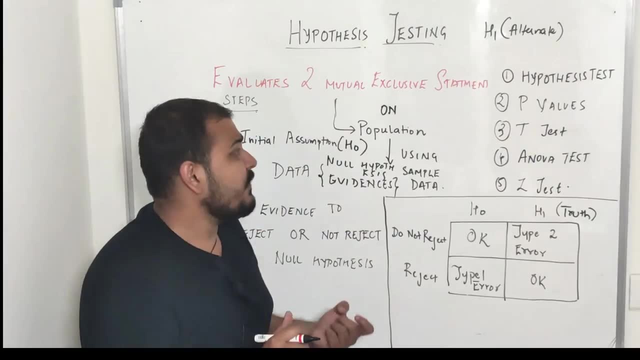 Lot of tests will be there for that. Okay, Now, you have understood this. Okay, Now, if I just consider, if I just consider this particular stuff and if I just consider that, suppose, if a Null Hypothesis is actually true, Okay, I am saying that. 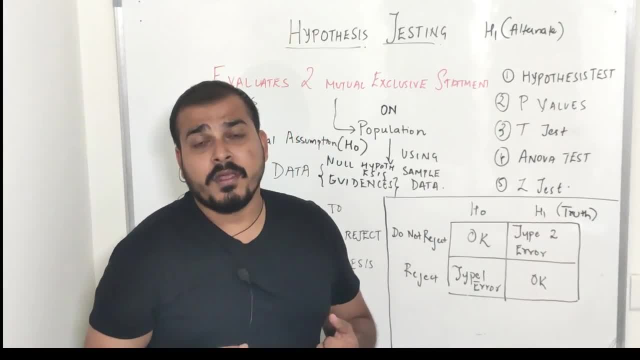 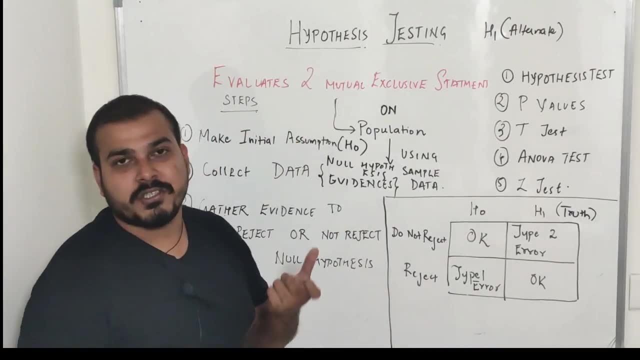 here the defendant is innocent, I am saying, But I don't have much evidence. I know somewhere or the other way this Null Hypothesis is true, but I don't have enough evidence. Then what will happen? This will get rejected, Right. 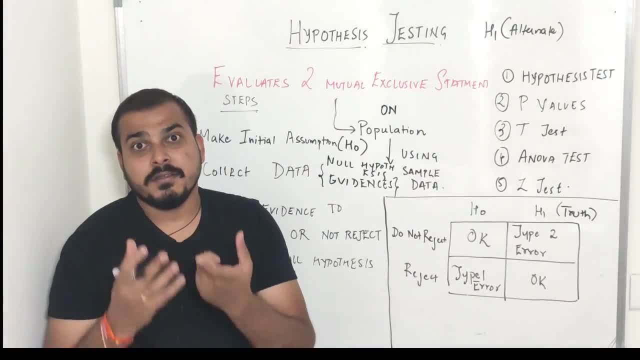 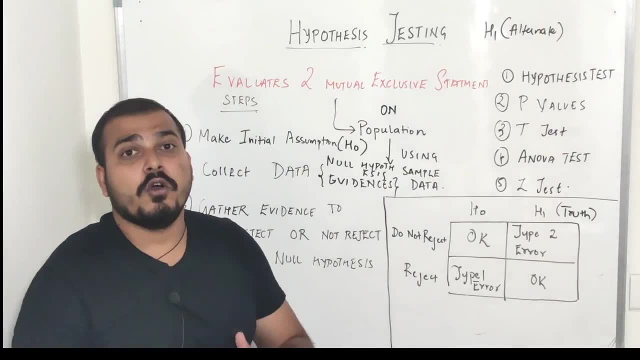 This Null Hypothesis will get rejected because I don't have much evidence, So instead it will get selected as Alternate Hypothesis. There the defendant will be true, He will be pledged guilty, But I know, or we know, suppose this defendant is innocent. 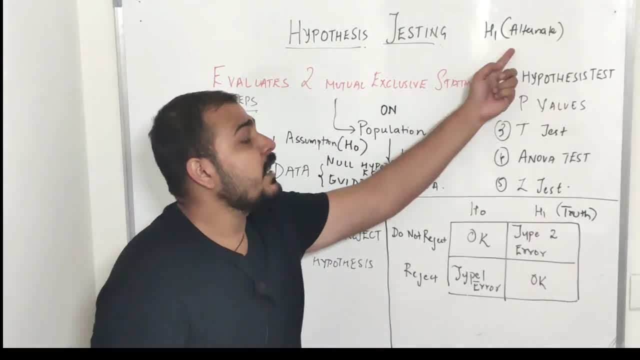 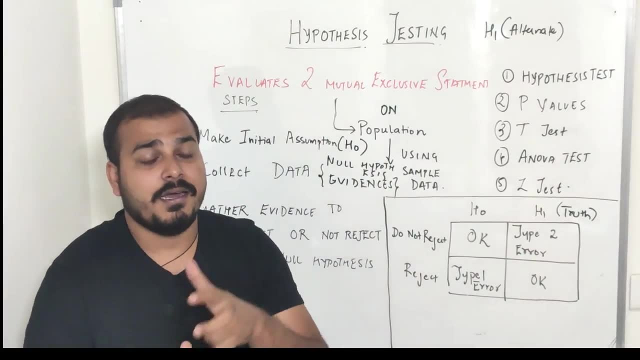 Right, And since we do not have much evidence, we are treating him as guilty. Okay, And if I go to this confusion matrix, I hope you remember if you know about classification, any algorithms with respect to classification. you have heard of confusion matrix. Now, in the confusion matrix in the top side, 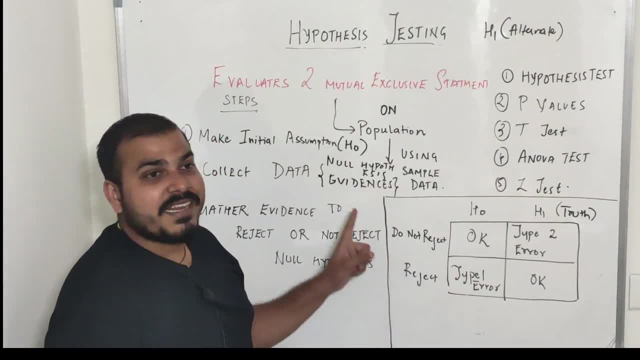 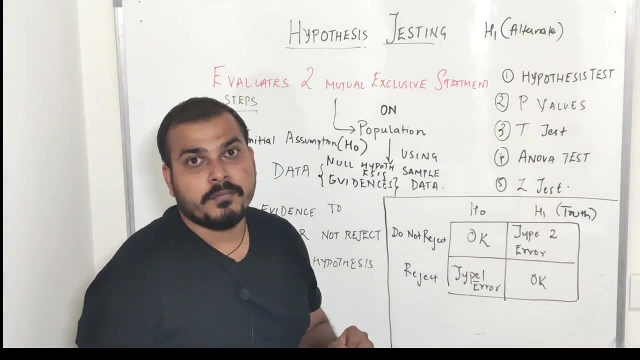 you have truth In the left side. you basically say that: do we have to reject this assumption? that is your Null Hypothesis. Or we should reject, or we should not reject. Okay, Now, in this particular case, I am saying that H0, my defendant is innocent. 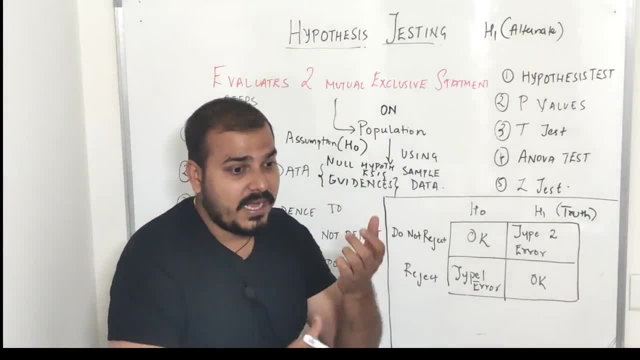 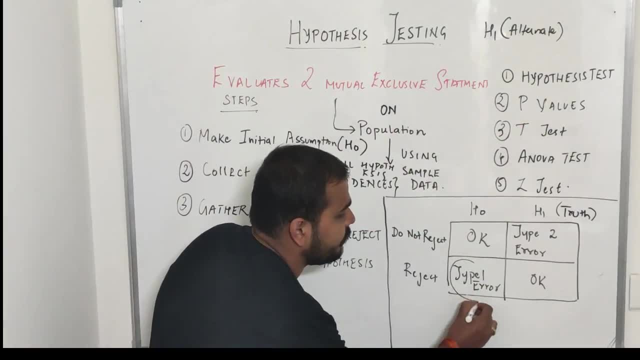 But I did not have. you know, I did not have evidence. Because of that, this got rejected and this got selected. Now this scenario will come over here, Which is basically called as my Type 1 error. Okay, Due to the lack of evidence, 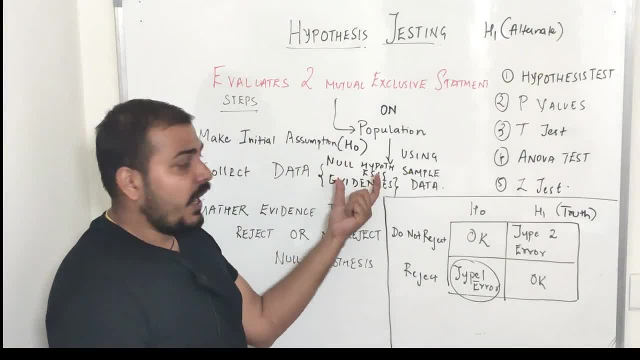 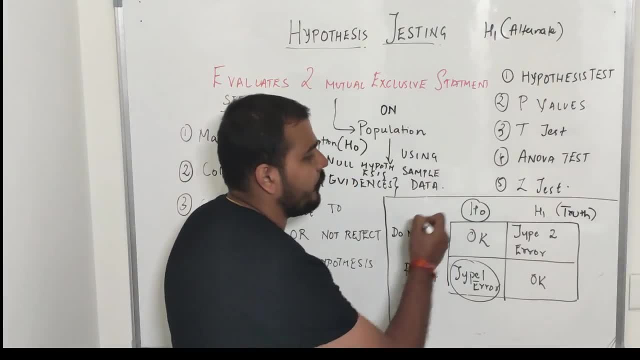 I had to reject the Null Hypothesis And because of that this is basically an error And because of that I have selected the Alternate Hypothesis. You can see over here this is my H0. Right, So this situation may lead to. 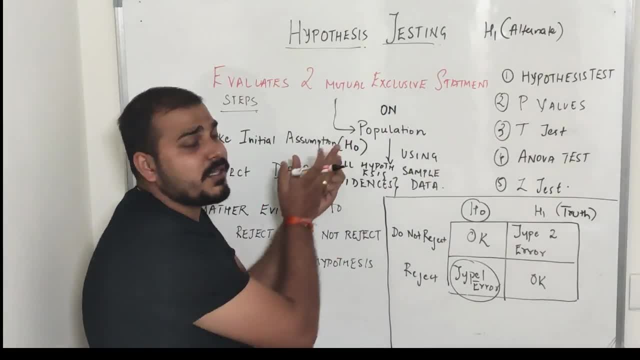 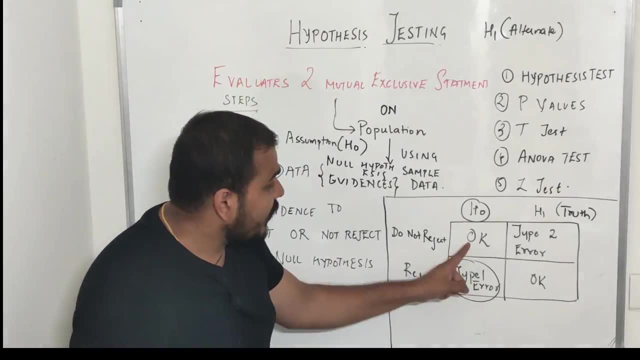 a lot of effect, You know, Since we know that this person was innocent But due to lack of evidence, we had to go over here, And this is what Type 1 error is actually belonging to. We know that this is true, positive, true, negative. 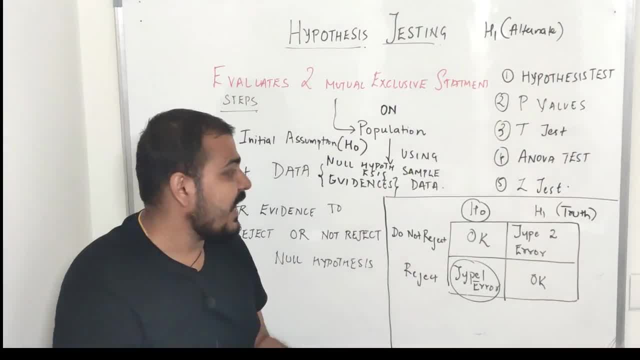 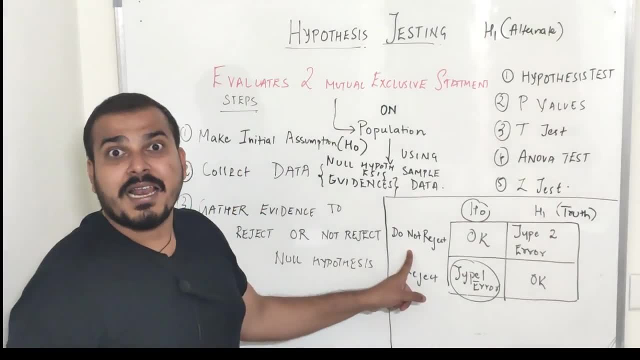 false positive, false negative, Right, I hope you all know this. This is confusion matrix. But what is the exact thing? Here we have the truth value. Here we have the Null Hypothesis. Here we have. should we reject this Null Hypothesis or not? 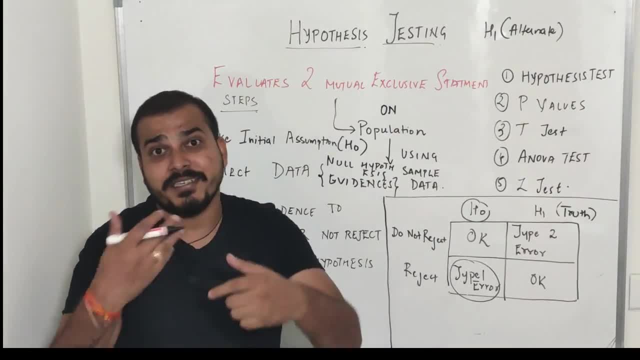 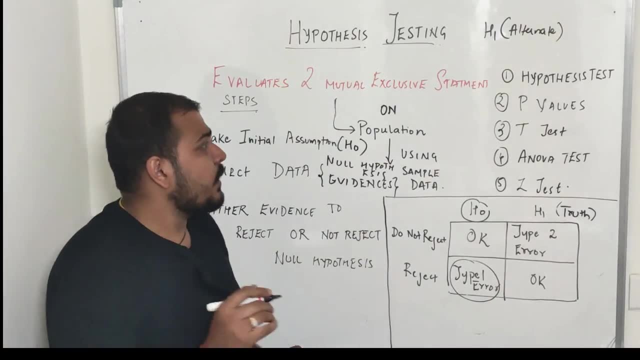 Or should we? I mean, should we reject or should we not reject the Null Hypothesis? Okay, So pretty much simple. pretty much easy to understand. What about Type 2 error? Let me take an example. Suppose I say that my Null Hypothesis says H0. 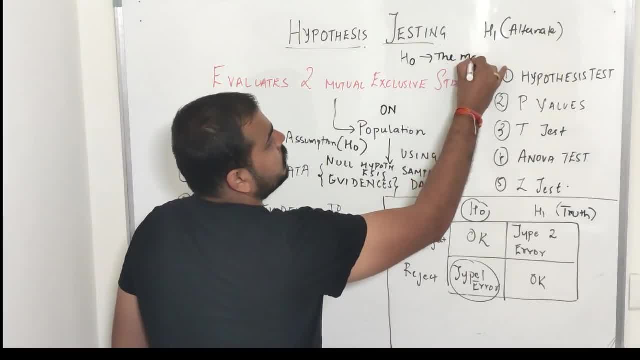 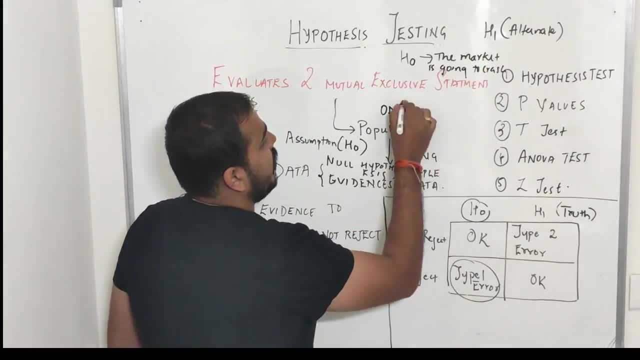 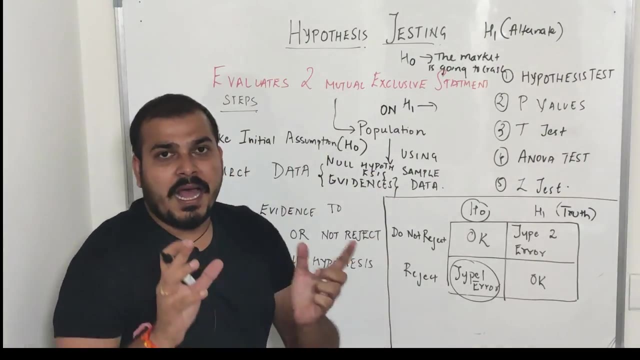 The market is going to crash. The market is going to crash, Okay, And my Alternate Hypothesis is the opposite of this. Okay, The market is not going to crash. Okay, Now what will happen? Suppose I do not have enough evidence now? 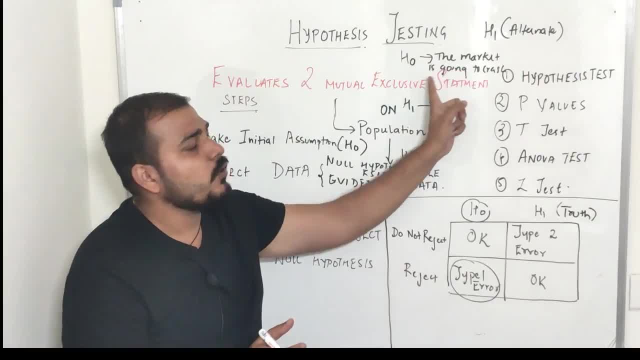 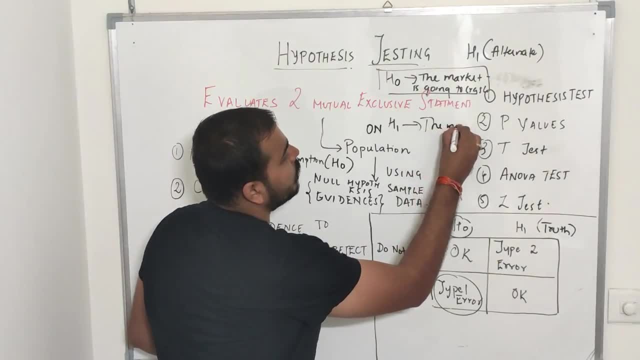 I do not have enough evidence. Because of this, I was not able to prove this market is going to crash or not. Now in my Alternate Hypothesis, suppose I say that the market is not going to crash. Market is not going to crash. 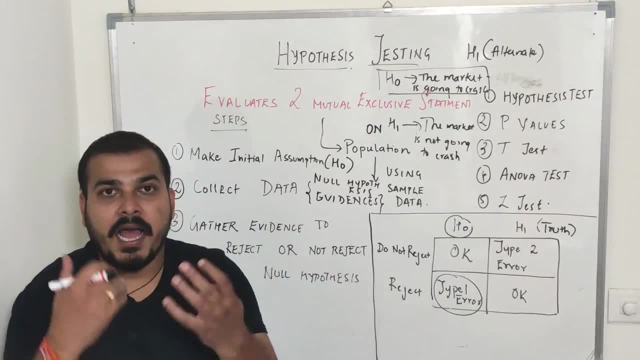 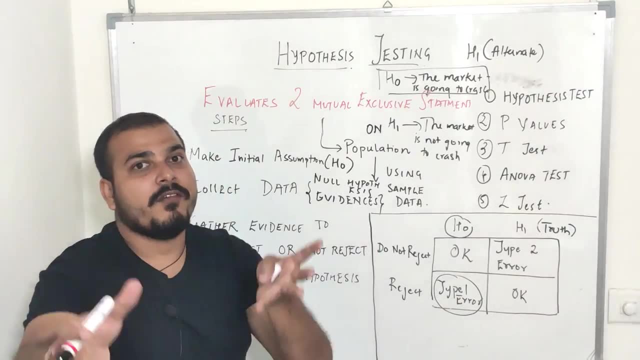 Okay And I collected various evidence. I collected various evidence And from that I found out that H1 became true. But suppose, due to some of lack of evidence, this is becoming true. The market is going to crash over there. So in this particular scenario, 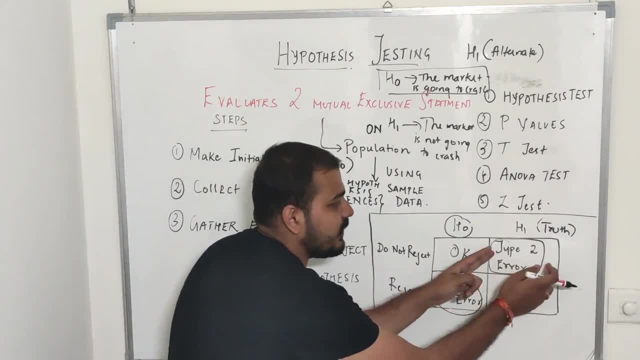 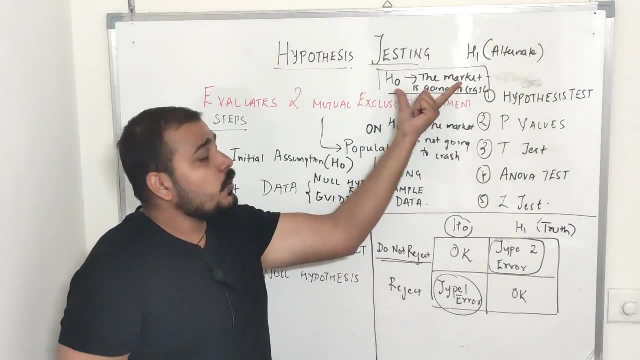 I will be getting a Type 2 error. Okay, And you can see that, with respect to this Type 2 error, I do not reject that Right. So this is basically a Type 2 error And because of this, we forgot to, or we. 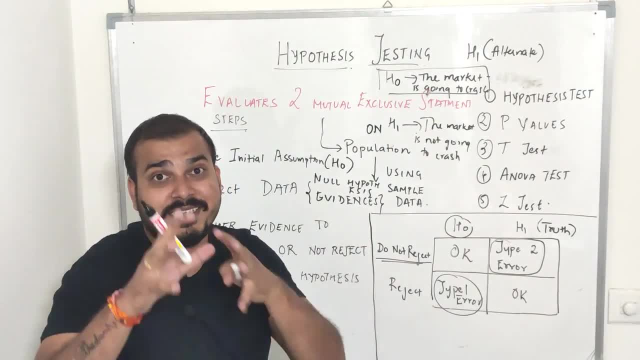 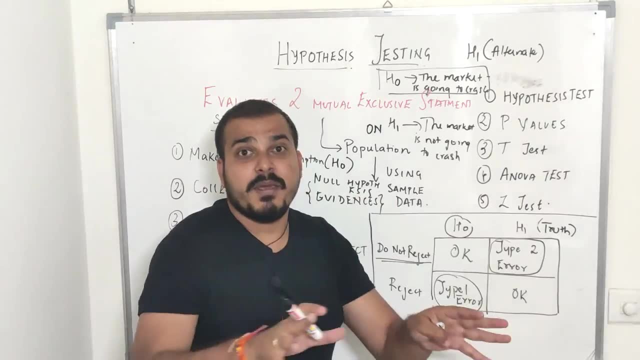 we did not manage to capture whether the market is going to crash or not. And this is catastrophic, guys, Because if we can understand if the market is going to crash, it can save a whole lot of money. It can save many people life Right. 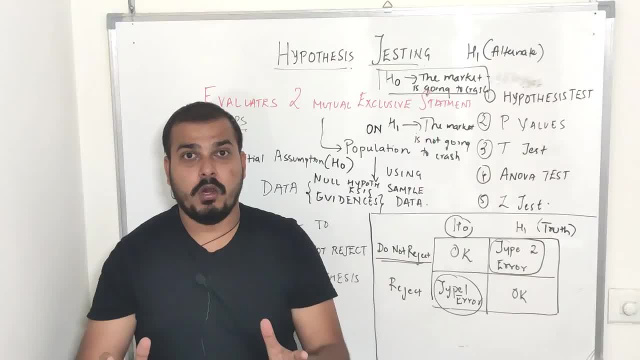 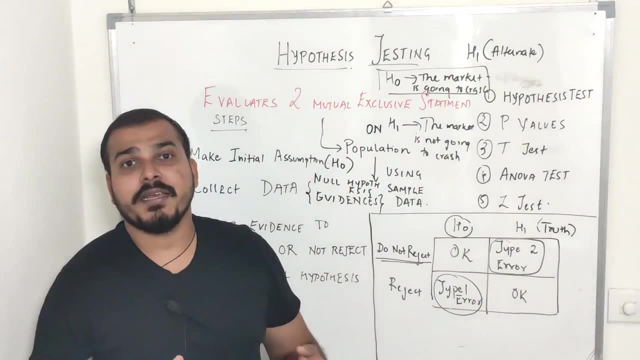 So this Type 1 and Type 2 error can play a major role in Hypothesis testing. So whenever you solve the classification problems, whenever you solve with the help of any machine learning algorithms, this always makes sure that you see this Type 1 and Type 2 error. 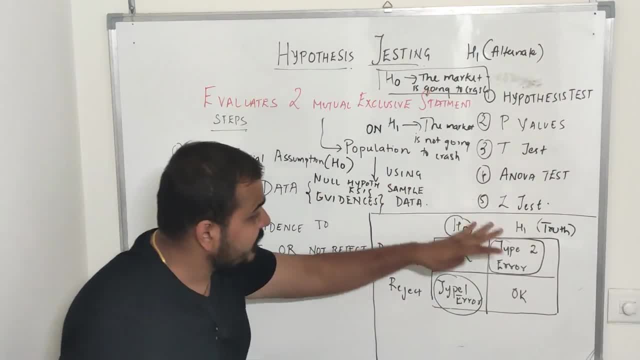 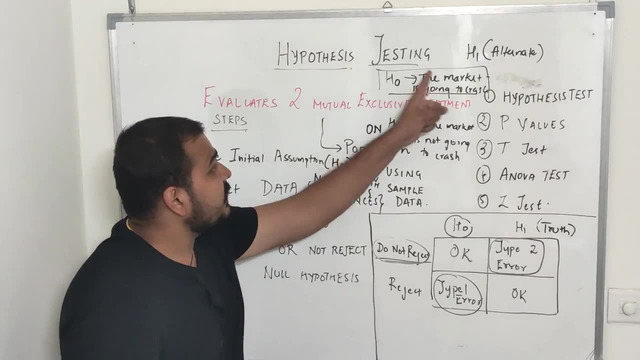 Pretty much simple, guys. Again, I am going to repeat what is exactly Type 2 error. Okay, Now here you can see that I do not reject this H1 statement, which is the truth, And, considering this market is not going to crash, I am going to approve this. 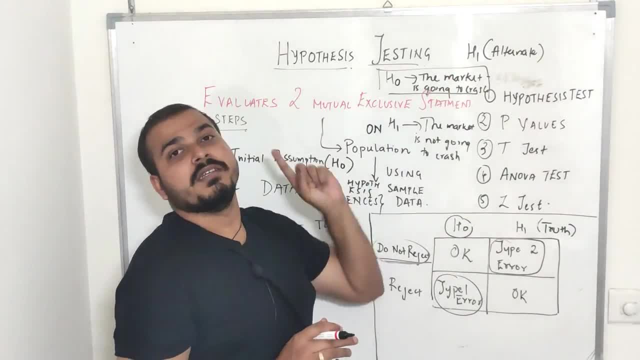 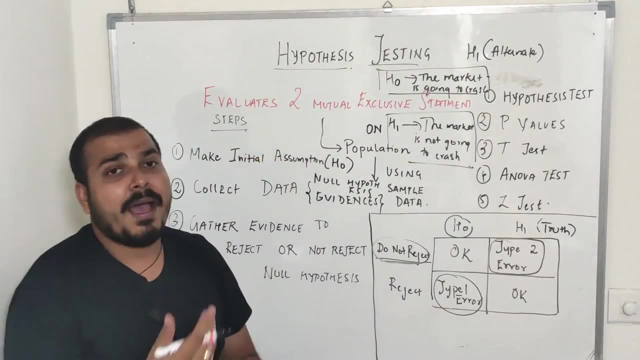 considering that I did not have much evidence to support this. Okay, When I did not have much evidence to support this, all I have to do is that I have to go and select this, But it may happen in such a way that, due to lack of evidence, in the future 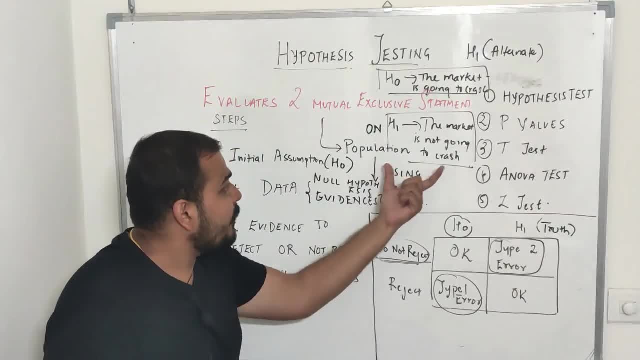 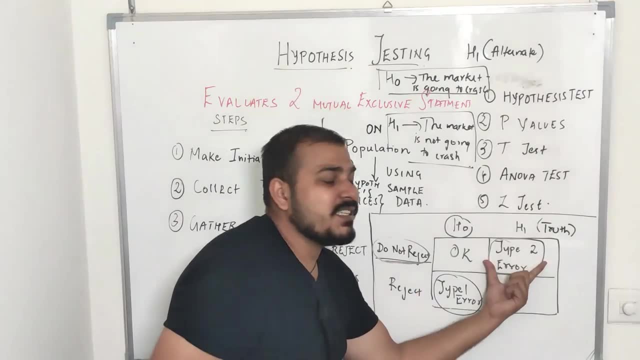 this was the original statement over there And because I predicted this, I came to a conclusion with respect to this Right, But when I tried to compare it with the truth value, this became my Type 2 error. So this is very, very important. 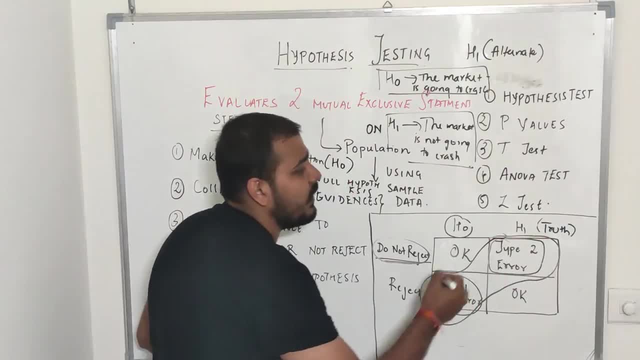 This Type 1 and Type 2 error to understand. Okay, And you should understand, with respect to the confusion matrix and considering the real world problem statement Right. So this is pretty much important, guys. This is what is all about hypothesis testing. 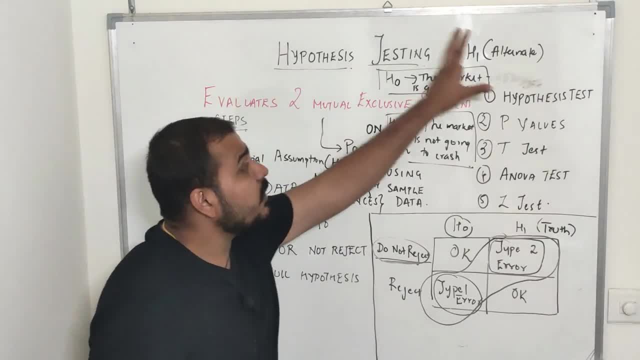 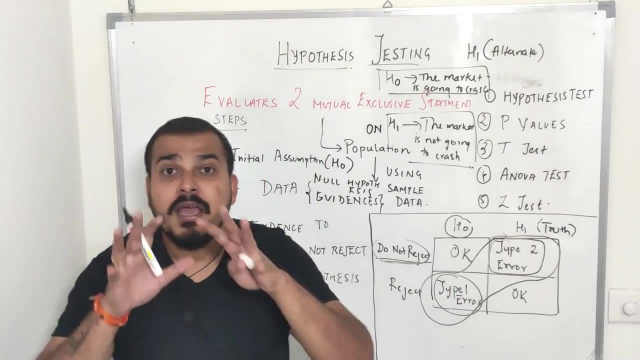 Okay, And it depends whether Type 1 error can be more harmful or Type 2 error can be more harmful, based on the problem statement that you are solving. Okay, And now, in my next video, I will be showing you how you can go ahead. 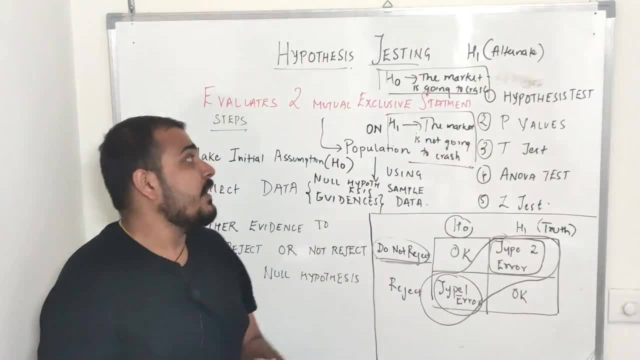 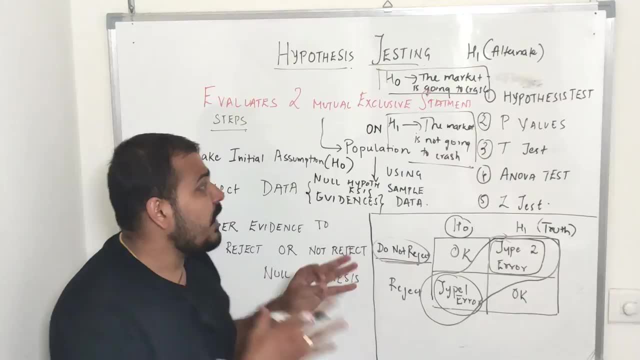 with hypothesis testing. How to perform hypothesis testing. How to perform hypothesis testing. Okay, And now, in my next video, I will be showing you how you can go ahead with hypothesis testing, How to perform hypothesis testing. I will be solving a simple math problem statement. 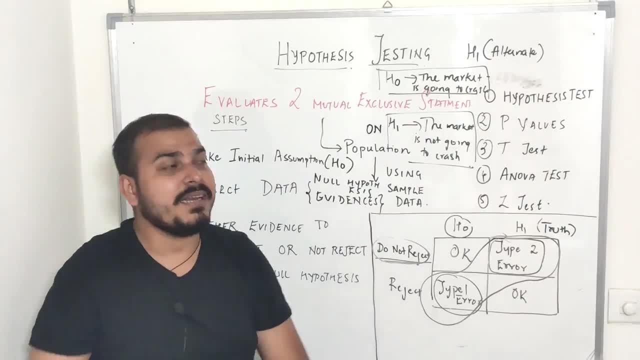 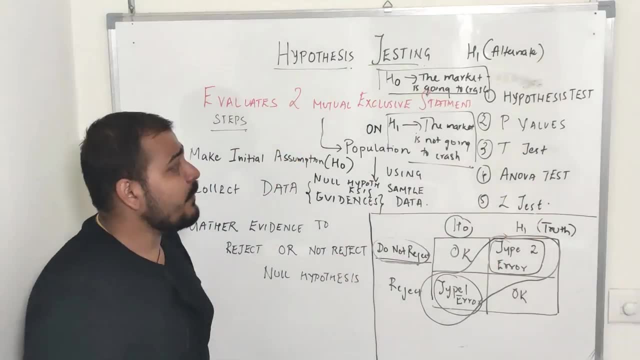 like how we did in schools, in colleges, so that you will be able to understand how to solve hypothesis testing with the help of P values. What is P values? What is T test, ANOVA test, Z test? Now, whenever I am saying that, 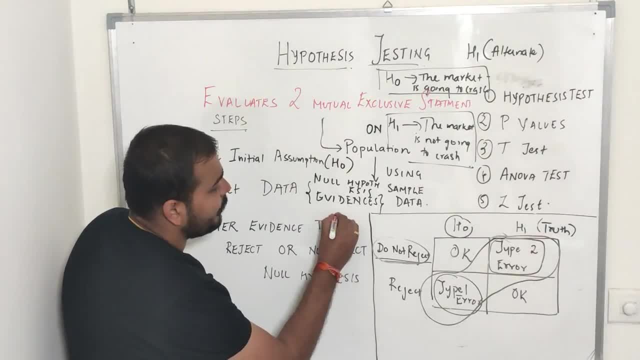 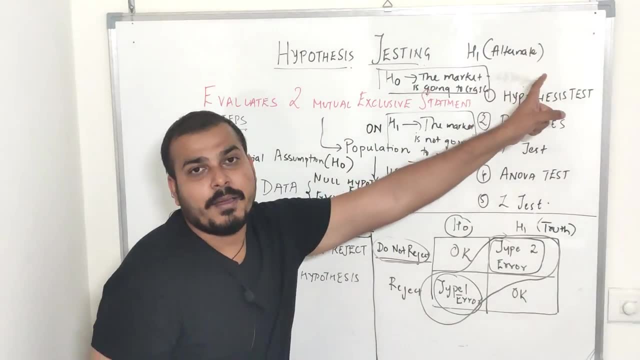 I am not able to prove this null hypothesis. we basically consider a P value less than 0.05.. If the value is less than 0.05, we reject the null hypothesis. go with alternate hypothesis. Now you may be considering: what is this 0.05??